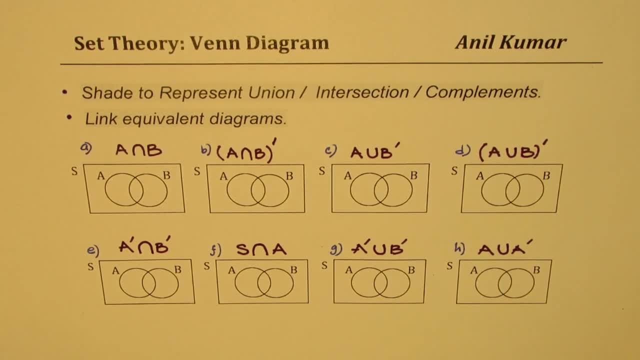 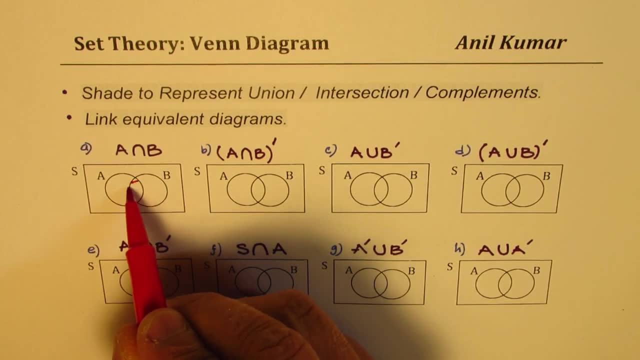 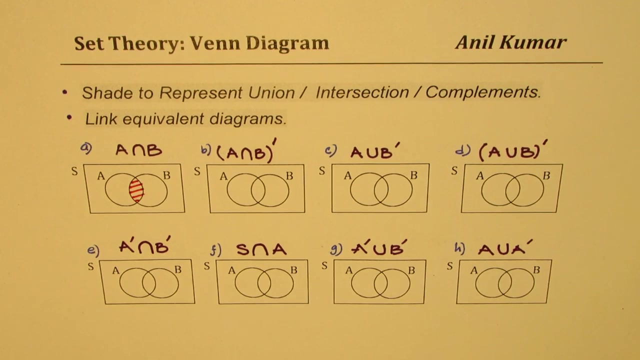 Okay. So let's begin with the very first one, which says A intersection B, which means common to both The region. common to both is right there, right. So this is common to both, Simple. The next one here is complement of intersection of A and B. This complement, that bar or a dash here, means not what is inside. 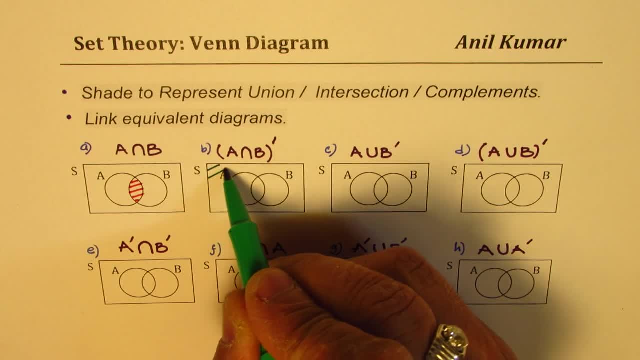 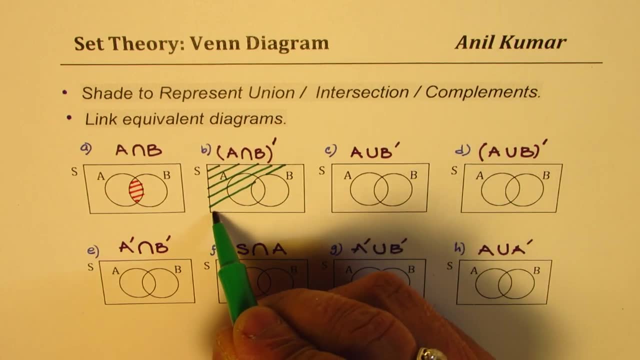 So not, what is this? That means everything outside, right? So let me just shade everything outside and I'll not shade anything which is common to both. right? That is the whole idea, right? So you have to stop here and then continue from that. 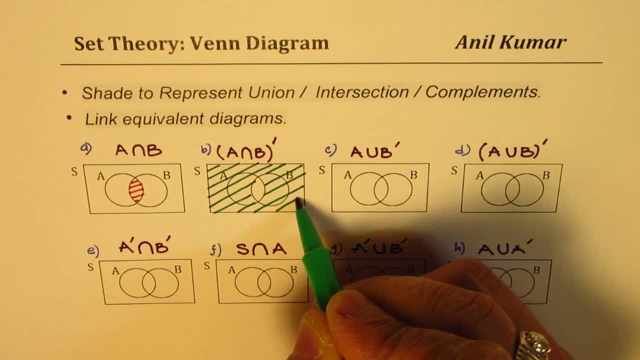 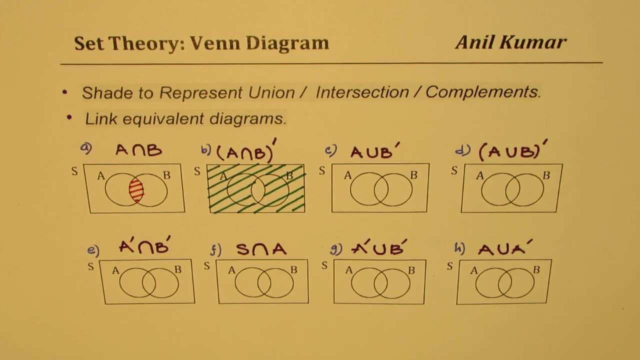 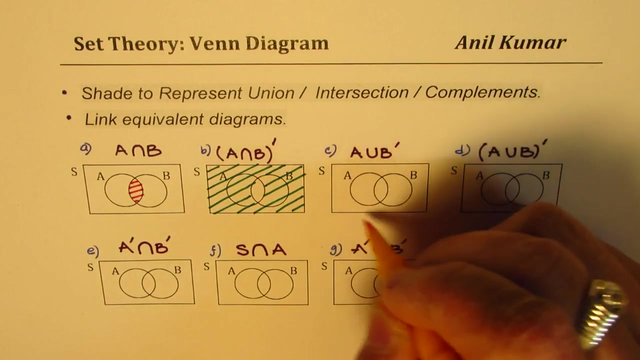 So that is Complement of A, intersection B. Now we get to slightly critical one. We're trying to combine union of set A with complement of B. So let's try to see what we're trying to do here. So when I say union means we have to combine, So not B means everything outside. 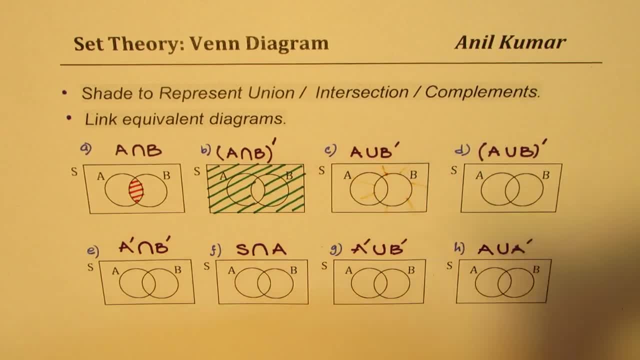 Do you see that? Not B is this? I'm purposely using Something which is not very bright, So it's not going to really damage whatever we are doing, but it will help us to understand. So that means not B, but all what is A right. 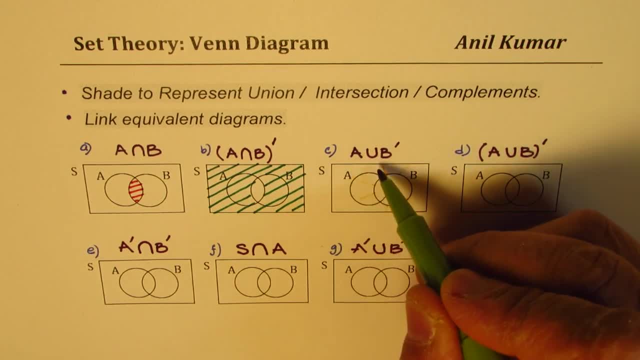 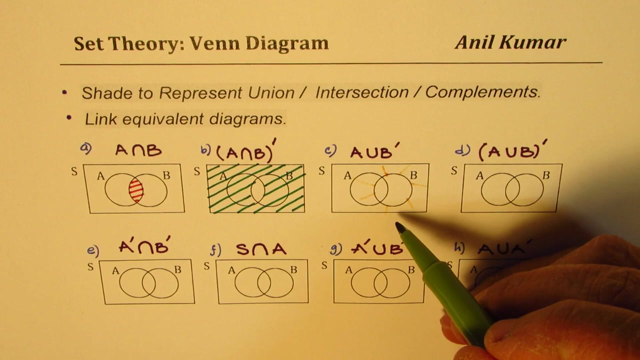 So we want everything which is A union, not B, right, So that is what we mean. So A is all this and not B is everything outside. So that means The only portion which we do not have to shade is this portion, because A is what 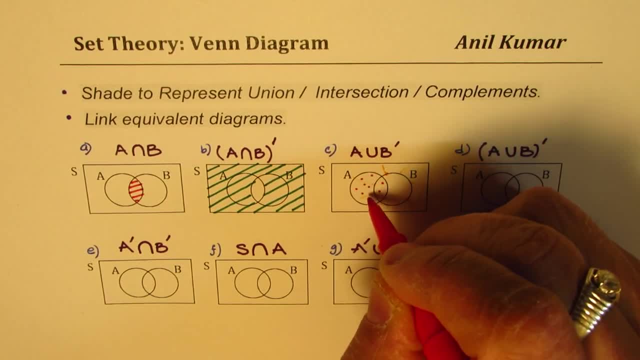 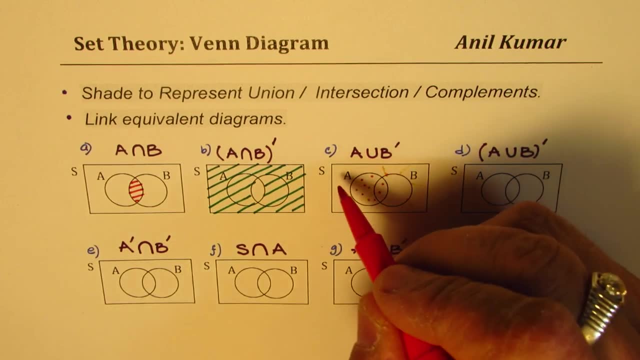 A is all this right, And so only that portion remains. So what we are going to shade now is everything here which is not B Perfect And also A correct, Correct. So that is what is being shaded. 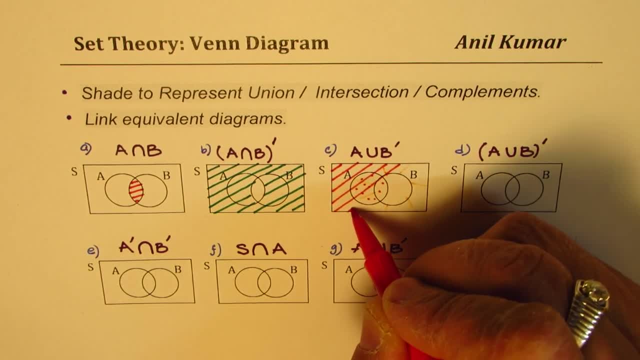 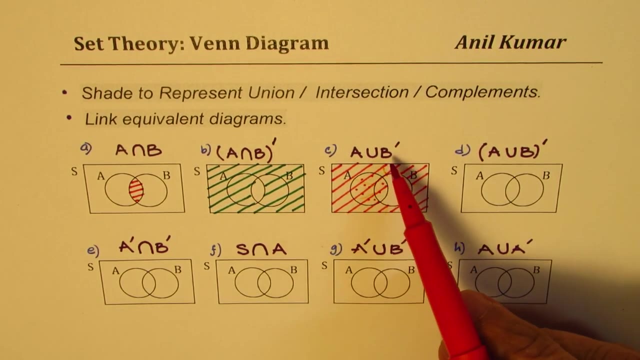 So I hope that is clear, But we'll leave this portion. You get an idea right, So that is how we are going to shade it. So this is union of A and complement B, Perfect. The next one here is: we have to see what is union of A and B and its complement. 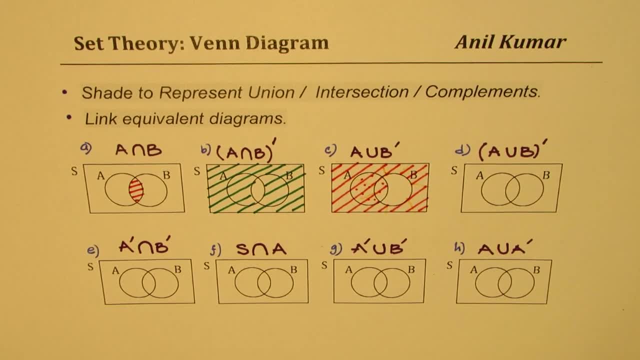 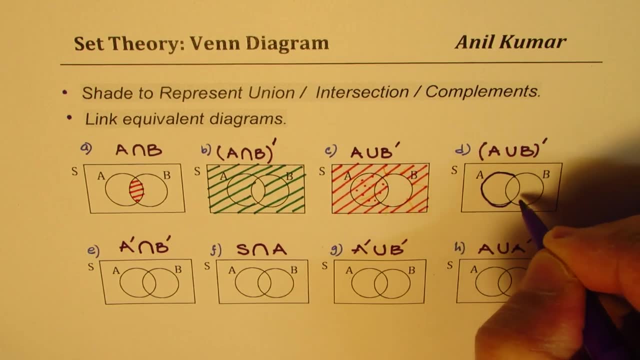 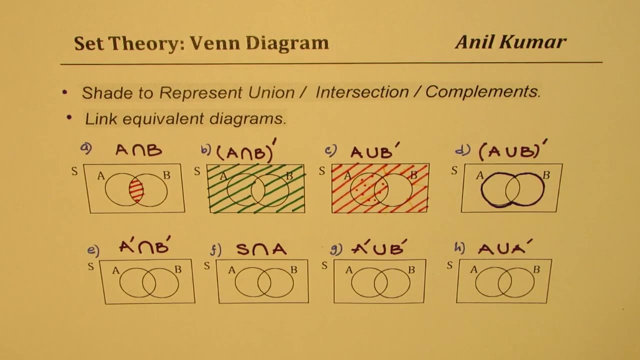 It means not Union of A and B, It really means not inside this portion. So let me mark this boundary, So we'll shade outside this boundary. We don't want this right. So everything outside this is going to be shaded now. 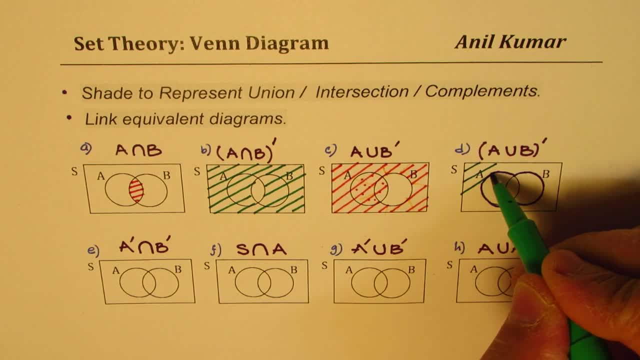 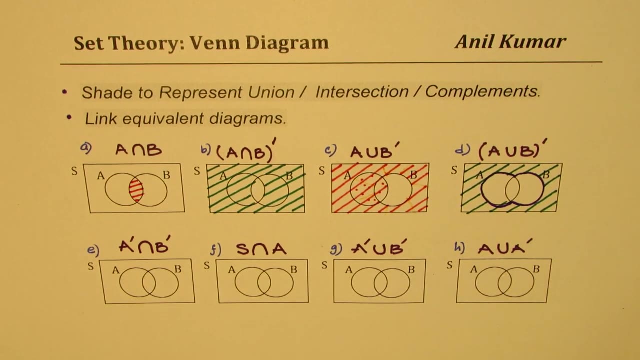 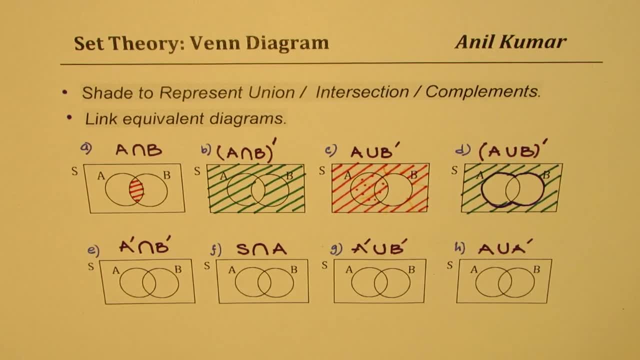 I'll like you to pause the video, Shade the other four and then check with my solutions. right, Let's look into the next one, which is very interesting. We need to find intersection of what is not A and which is not B. 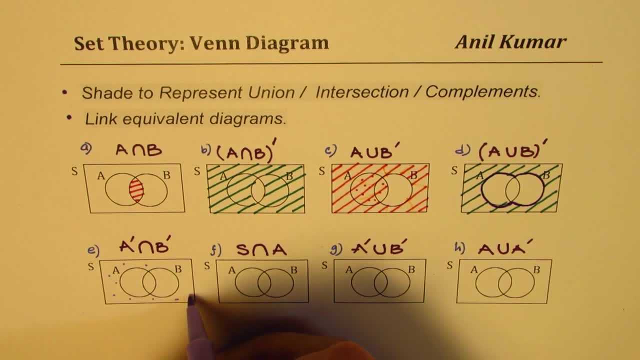 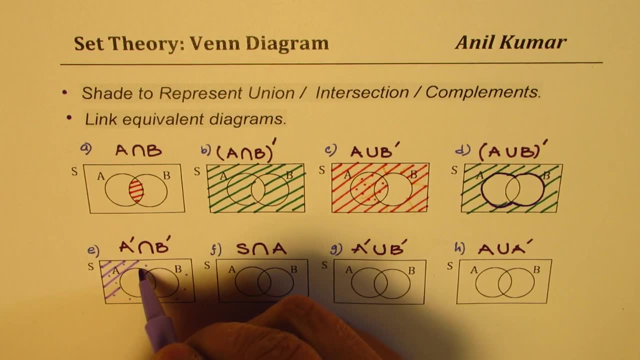 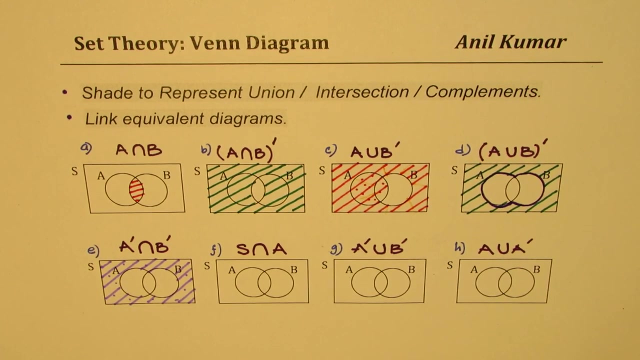 Yeah, Yes, Yeah, Yeah. A and B. Do you get the idea? So that is what it is, So let's share it. Okay, So that is intersection of not A and not B. Now we are not comparing with the universal set. 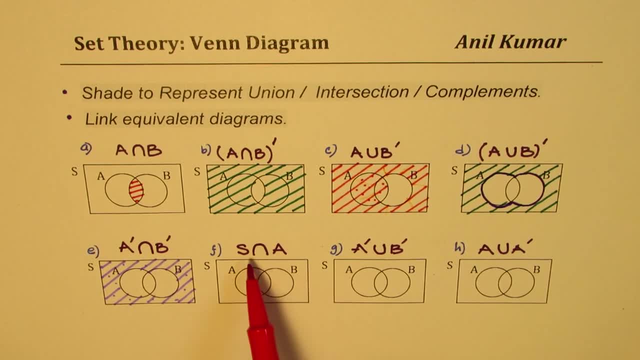 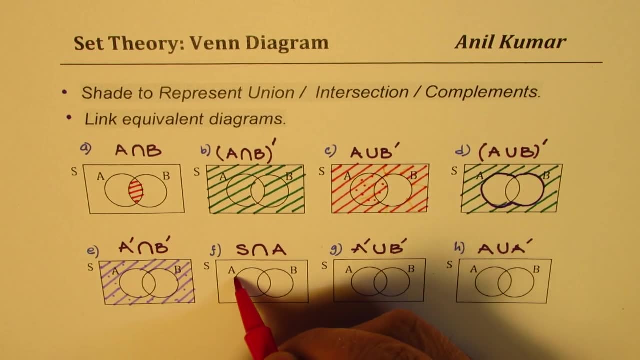 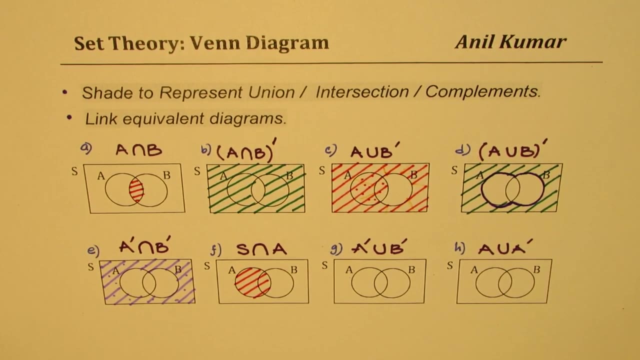 and we want subset, I mean intersection of A with the universal set. So that means the set A itself. right, So that is the set A. The next one here is union of not A and not B, right So? 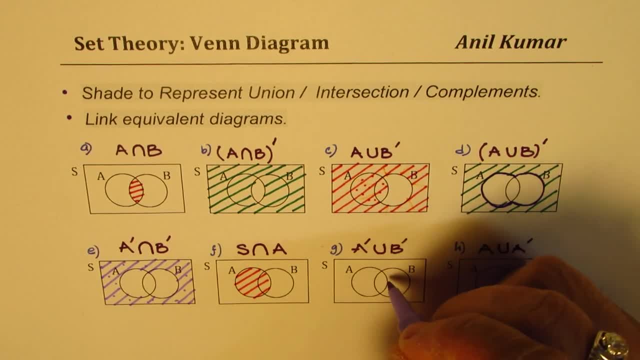 not A. let's use dots. Not A means everything outside. Do you see that, Not A? So everything outside is not A, And what is not B Not B is everything outside like this. Do you see that That is not B? 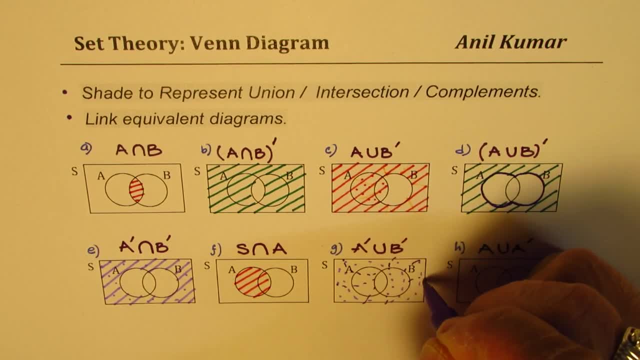 everything outside B. So that means if I leave this portion which is common to both A and B, I should shade rest of A. So that is what I am going to do. So that is what it is Right. So with the help of Venn diagrams we can actually prove many identities based on set. 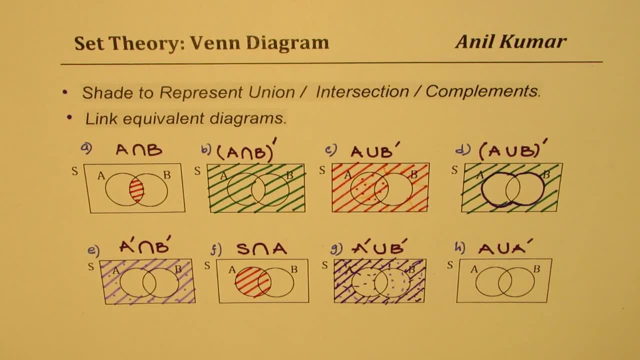 unions, intersections and complements, Perfect. The last one here is union of A and its complement. You know, union of A and its complement is the whole universal set, right? So it is everything here Perfect. So you find that this is equal to the universal set S and this is equal to. 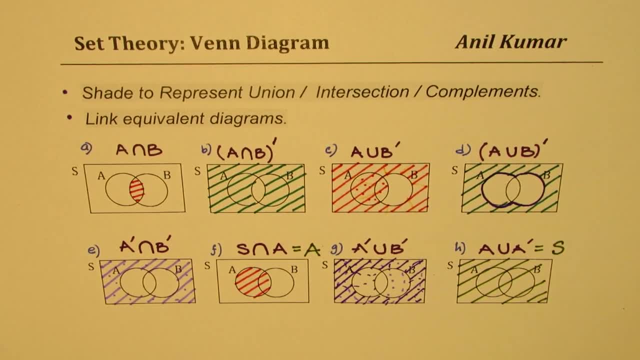 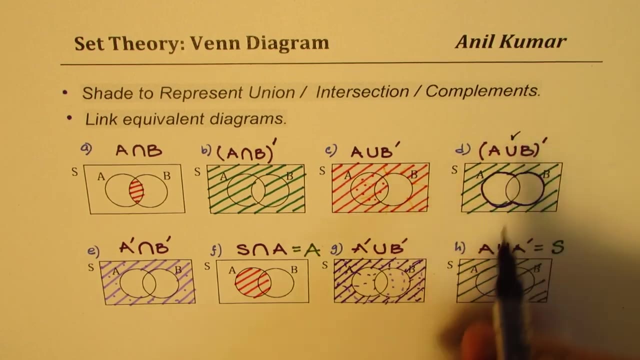 the set A. Can you find some other sets which are equivalent? Watch carefully and then write down your answers. So what do you notice here is that, what is this? equivalent to? D, which is A union, B complement. So that means everything outside A and B. it is equivalent to the. 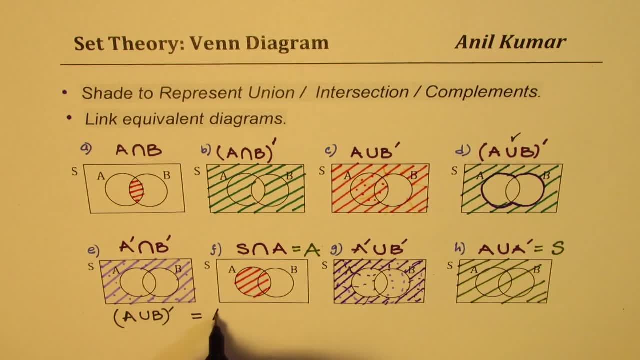 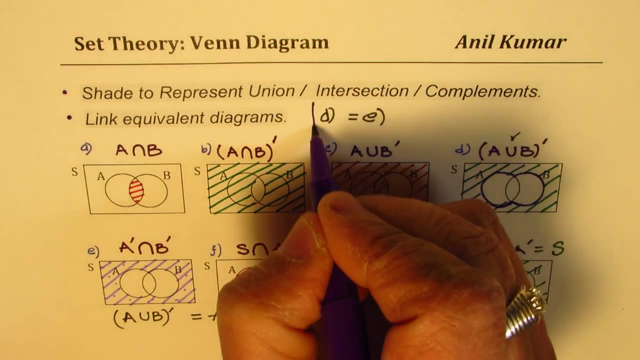 intersection of not A and B. Do you see that It is equivalent to the intersection of not A and B, right? So that is one relation which you see. You find that D is equal to E, right? So that is one thing which you notice. Now you can actually prove it. 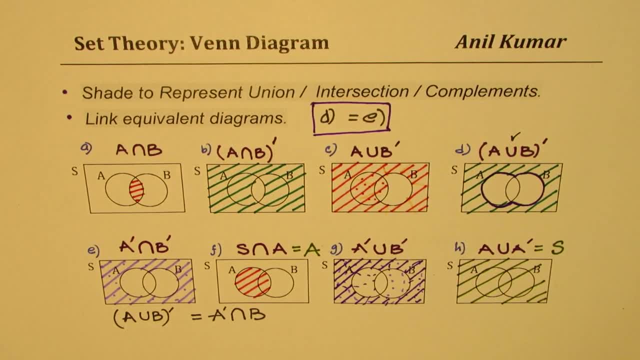 algebrically also. I'll provide you with a link which will help you to understand how to prove this algebrically. Got it? Do you find any other interesting things which are related? Right? So here, while I was shading, I didn't shade this. I have to only leave that portion. 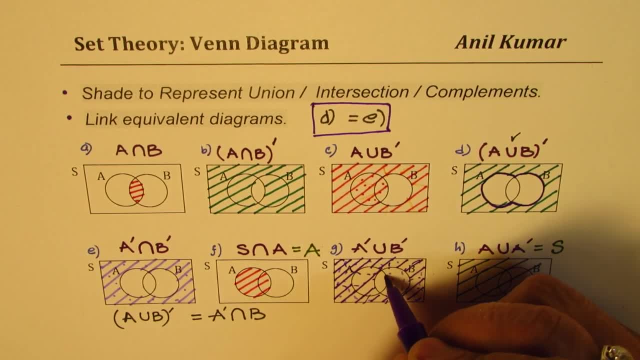 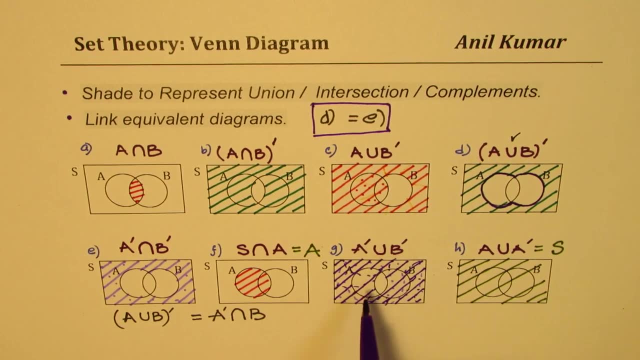 right, So this should have been shaded. Good, I saw it right. So, okay, When we said union of not A and not B, we marked this right. Those dots means it was marked correct, So not inside the intersection. That is what it means. So basically, 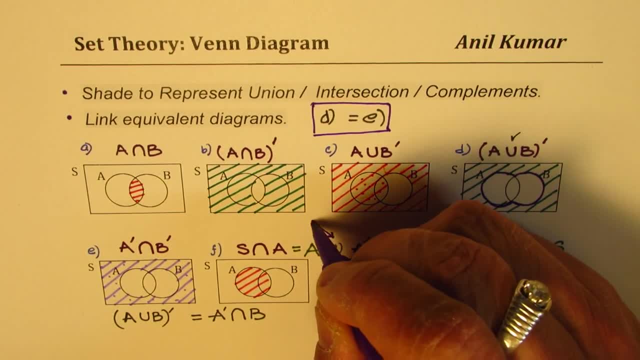 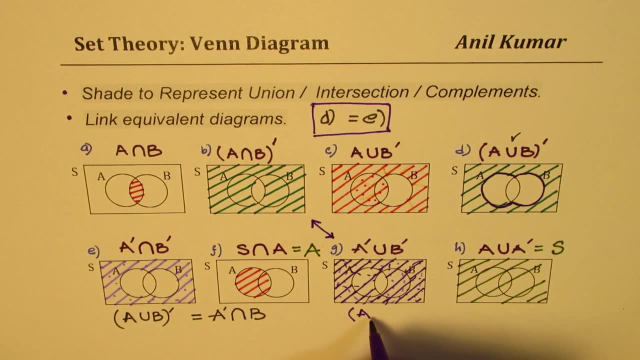 you see that these two are also related, Got it? So from here, what we notice is that the intersection of A and B and its complement is equal to the union of complements of A and B, correct? So that is another important relation which we see from here. So we find that B 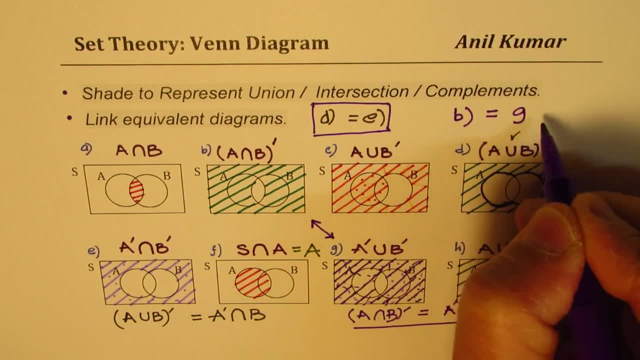 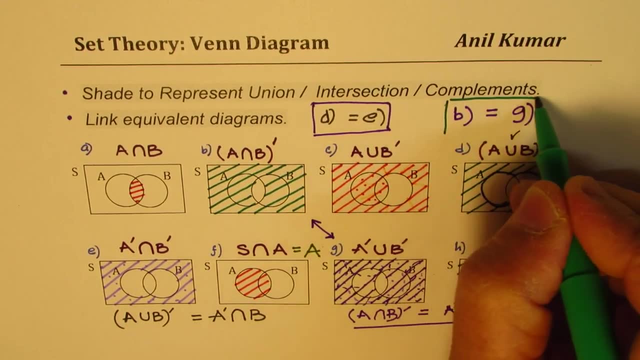 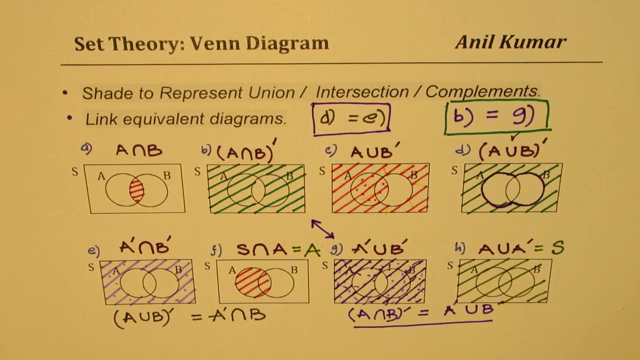 is basically equal to G, correct? So that is another relation which you see from these diagrams by shading. Instead, take it as an exercise to prove this algebrically perfect, And you can always watch my videos for the complete proof. I hope that really helps. So I'll take up another. 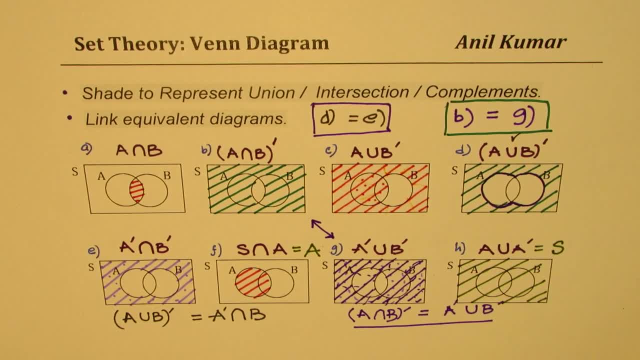 quiz for you based on what we have done with a twist to it, and let's see if you really understood the topic. Feel free to write your comments and share your views, if you like, and subscribe to my videos. That'd be great. Thanks for watching and all the best to you. 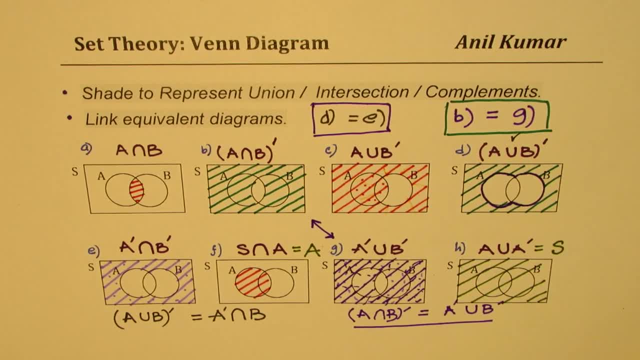 Bye-bye Subtitles by the Amaraorg community.